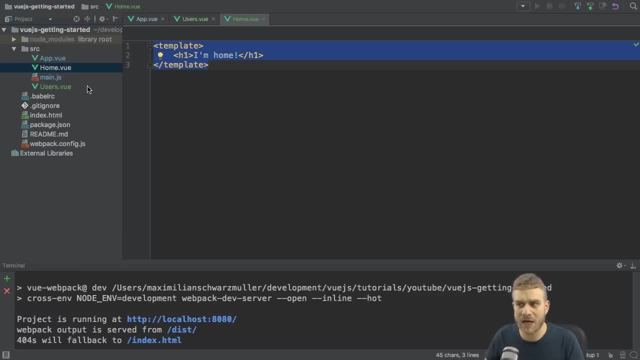 Home and users, and in both I only say I'm home and users overview, But I think we can easily imagine that we would have some users in there or generally some different components you want to load conditionally through routing. Now why would you want to use routing in the future? 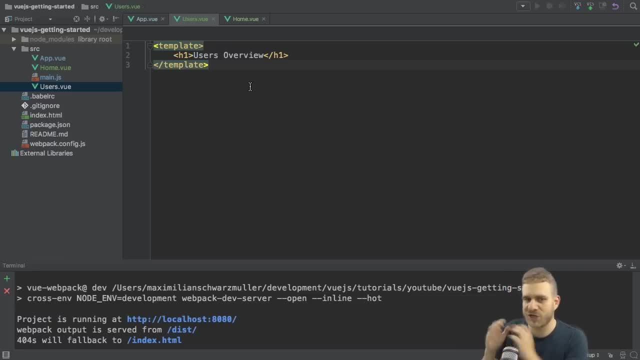 First place there is the if and so on. if you want to conditionally show certain components, right, Well, routing is of course useful. if you want to create a single page application, That means the only page ever getting served by your server is the indexhtml file, this file here. 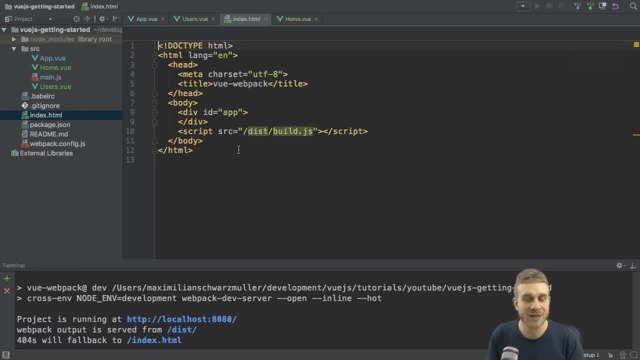 Now, in this file, we're loading the Vuejs application, but in this application, we maybe want to recreate this application-like feeling, this website feeling, where we do have different routes. Now, here, though, the routes will not be handled by our server. We're not sending the request to the server, We're not getting back multiple pages or views from the server. 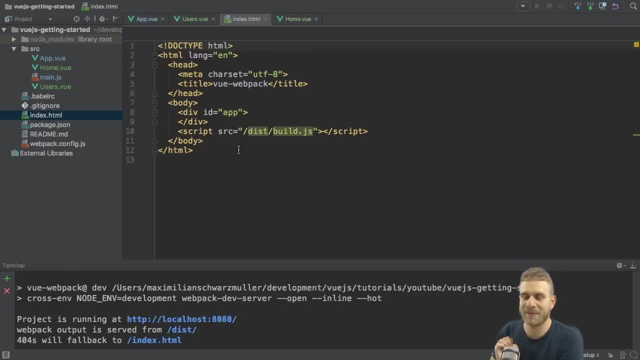 Instead, as I just mentioned, we're only getting back this indexhtml file. but we still want to handle different routes, And turns out we can do that with the Vuejs router, A nice little package we can add which allows us to parse that URL and load different components. 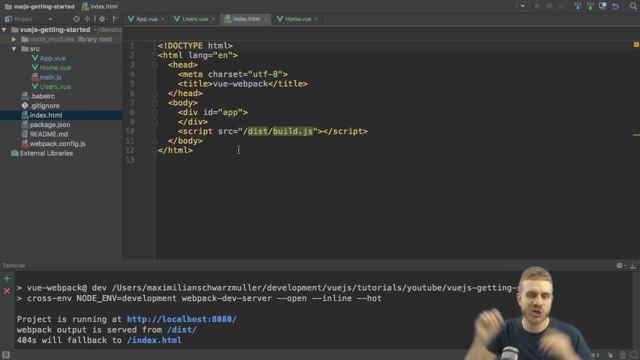 As pages, so to say, depending on which URL we're visiting. Now, in this video, we're going to have a look at how we can set up this router, how we can configure our basic routes and how we can go there. In the next video, I'll take a closer look at how we can navigate around and, especially important, how we can pass data when switching the route. 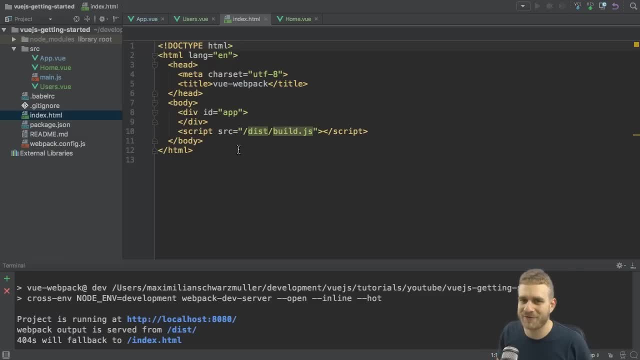 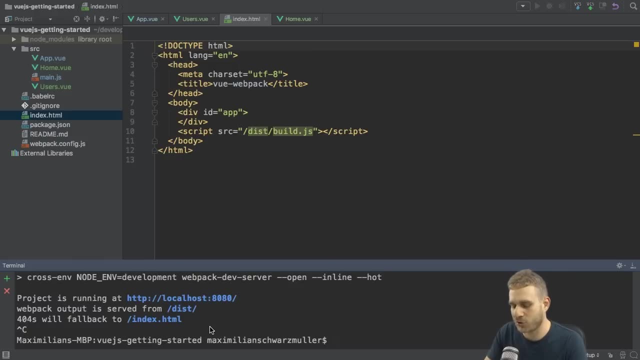 So enough of the talking, Let's start working on that router. I already got my development server running here And I'm going to cancel it by hitting save. And then I want to install that Vue router. That's an extra package. It's not included in the default Vuejs package. 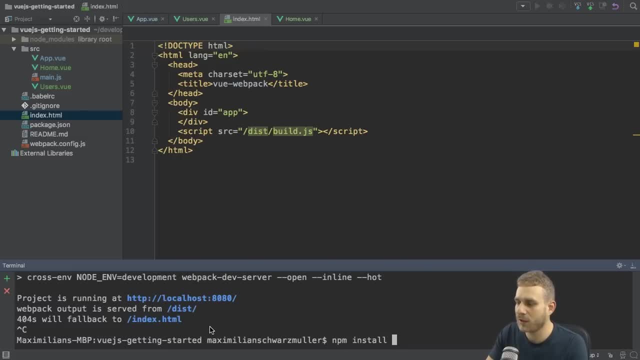 And we can install it running npm: install minus, minus, save to save it as a dependency in the packagejson file Vue router. This will pull down the router and make it available for us to use in this project. Now, with the router installed here, we can go to the mainjs file. 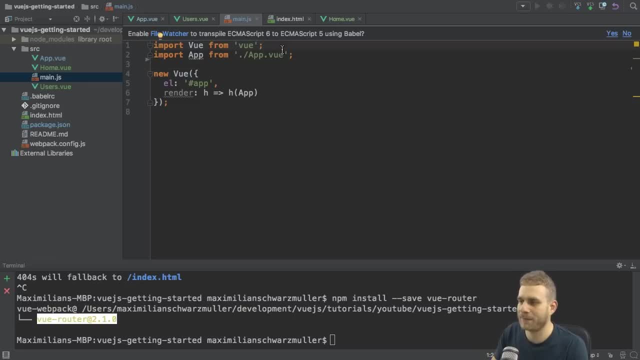 Which is our root entry point for that application, as you learned in the CLI video. if you watched that on this channel And here I can now import the Vue router. Now I can give it any name I want here, but I have to import that from Vue router like this: 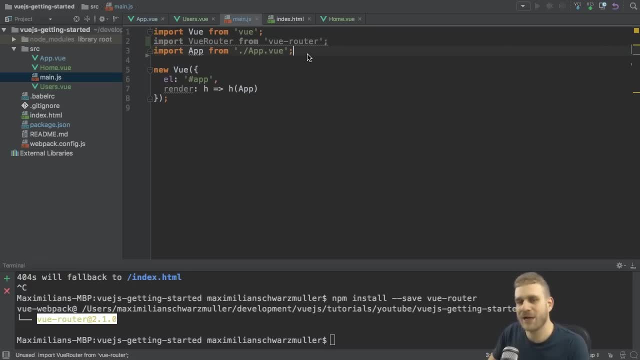 So now this will give me that router And in order to be able to use it here in this application where I'm using Webpack to bundle everything, I have to take my Vue object, Which I'm importing from Vue. So this root Vue, not instance, this Vue object really from the Vue package. 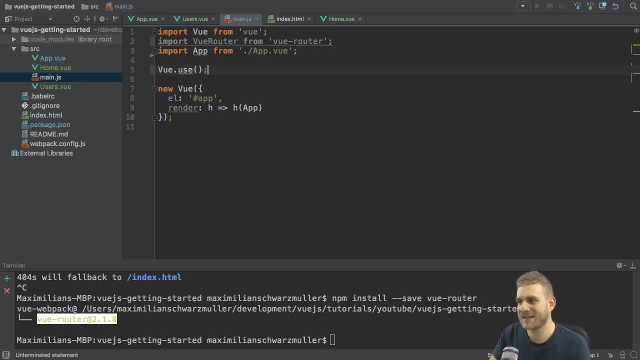 And execute the use method there. This enables plugins which I can use, and the router is just such a plugin. So by calling Vue use and passing the Vue router, I'm making sure that routing is now actually enabled and will work, So that now gives us access to the router. 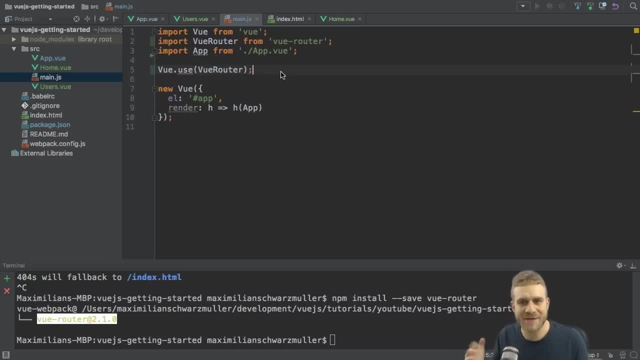 But we haven't got any routes to navigate to. We get the app- excuse me, we get the home and the uservue file, But how do we get there? Well, we need to set up our router. So let's add a new constant to the mainjs file. 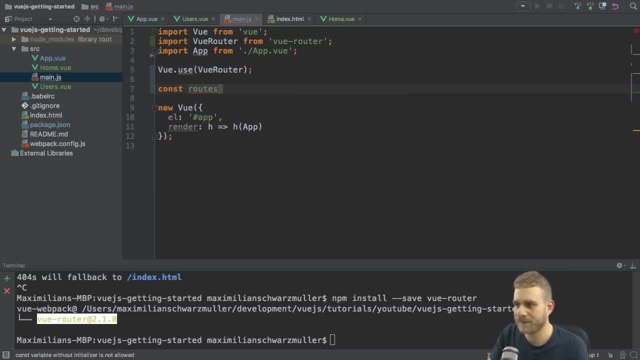 And let's call it routes, to set up some routes first. Now, routes is basically an array of routes. This, of course, leaves the question: how does one individual route look like? Well, one route is simply just a JavaScript object. So we configure a route by adding a JavaScript object to this array. 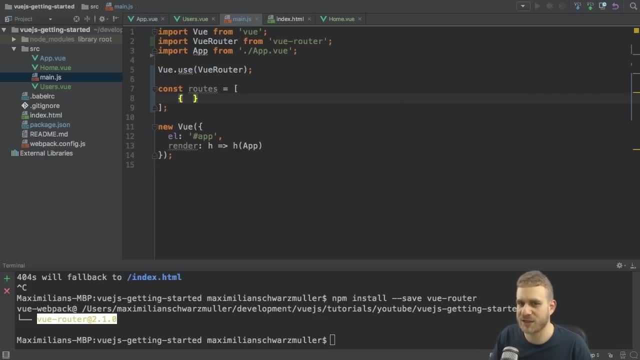 Now that array is not getting used anywhere, but we're going to change this soon. So, in order to set up a route here, we now need to define a path, And path- and this is important- refers to the part in our URL after our domain. 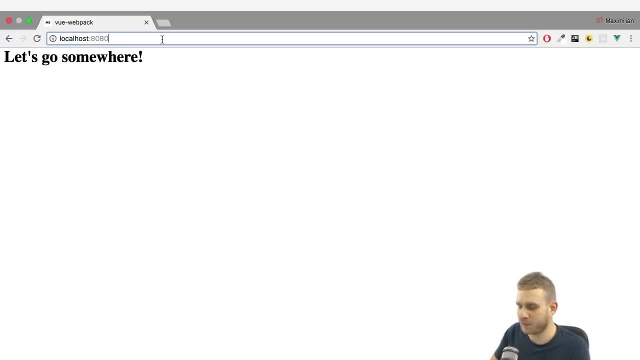 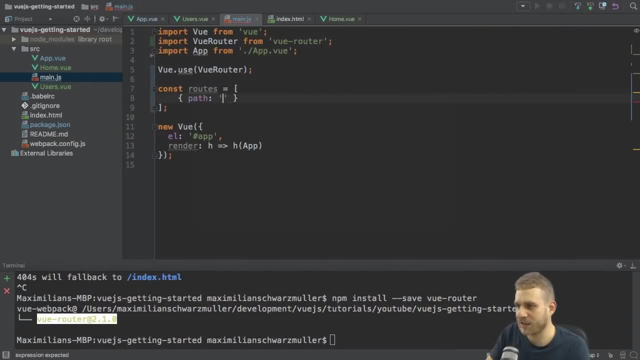 So here the domain is localhost 8080. And the path would then be, for example, slash users. That would be a path: slash users. So let's say we want to handle the slash users, So we add slash users here, And then we need to specify which component should get loaded. 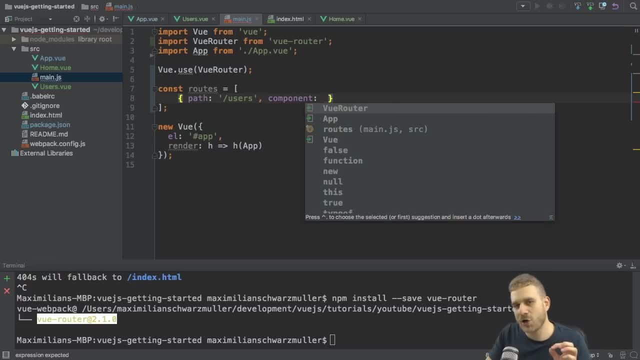 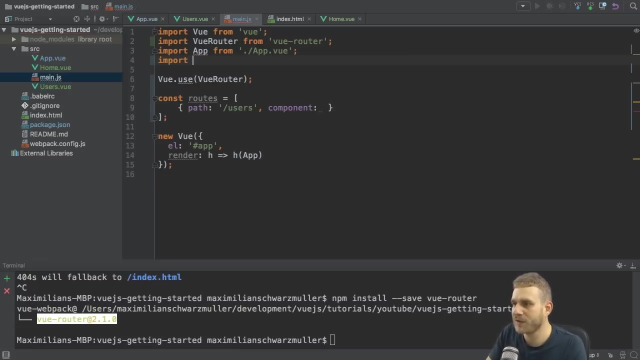 So component. Now here we can define which component we want to load. if the user navigates to localhost 8080, slash users. Now, if that shall be the users component from the usersvue file, we need to import that. So import users from usersvue. 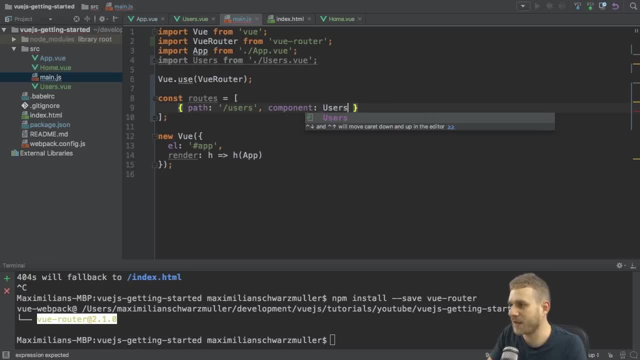 And here I simply set this up as a component. then Users: This gives me the users path. Now let's add another one. Let's add a default path, shall we? So that we always load the home component if we're just at localhost 8080.. 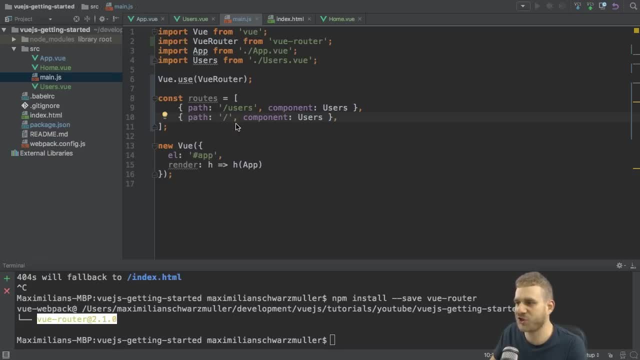 So for that I will just enter an empty path, just slash, And here I will duplicate this, And I want to load the homevue file, the home component, And therefore here the component is home. Now, with that I got two routes set up. 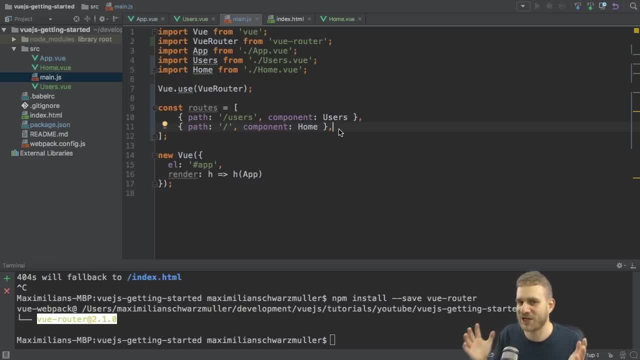 Users for slash users and home for just slash, for localhost 8080, in this case here. So we get the routes. This is certainly great, But how do we get the routes into our application now? Well, nothing easier than that. We simply create a new constant. 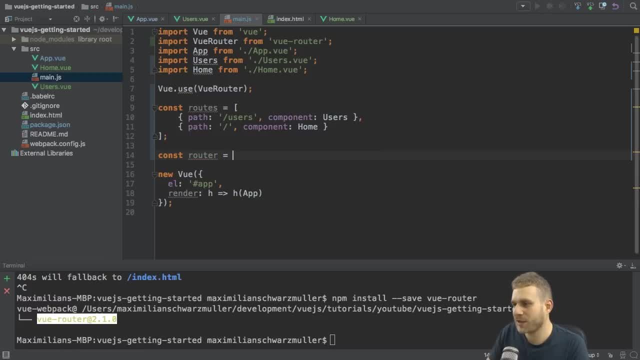 Let's call it router, And router now uses the Vue router, So new Vue router here. And we pass an option, Object, tuted, constructor. In this object I simply pass routes And I could say routes, colon routes, But since I'm using ES6 here, I can take the shortcut and just say routes. 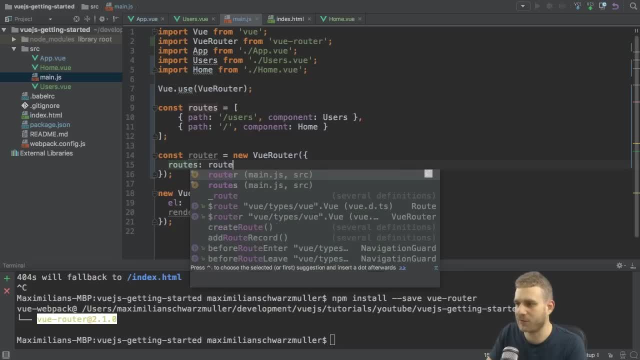 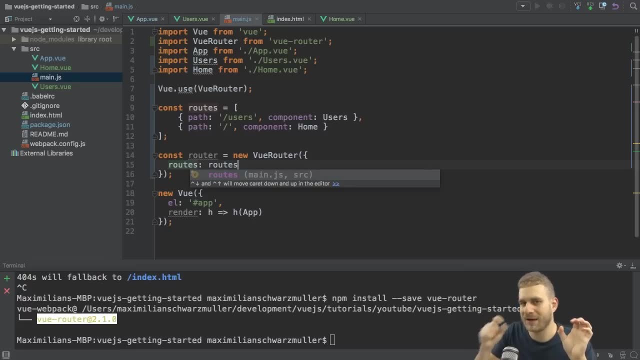 And ES6 will automatically expand this to routes routes. So that's just a shortcut in a case where the property name and the name of the value or the variable name which holds the value are equal. So if both are equal, we can leave out the value name. 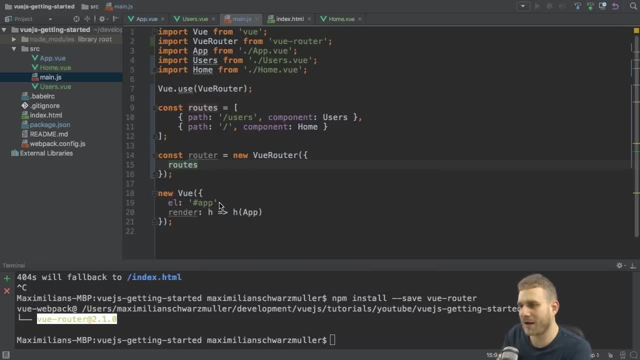 And just put routes here. This creates the router, And now we have to add this router to our root Vue instance By adding router, colon, router, Or again using the shortcut just router And let it expand automatically. With that the routes are set up. 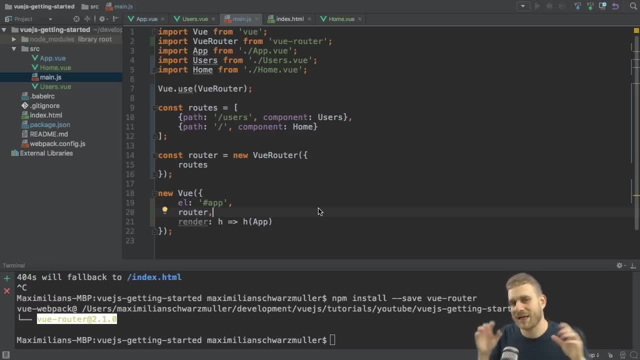 The router is set up. The router is also added as a plug into Vuejs. Almost everything has been done. Now we need a place to load these components at, Because right now, Yeah, we get slash users and slash registered as routes, But we don't have any place to load them right. 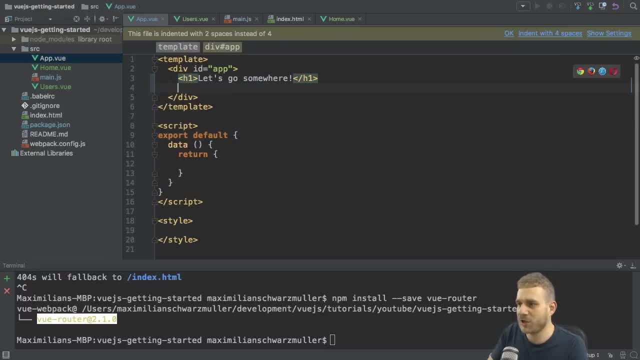 So let's go to the appvue file And here, in that template, We should define a place where Vuejs should render the routes we're navigating to. That is done by adding a router Vue. Now, router Vue is just a reserved component. you should say: 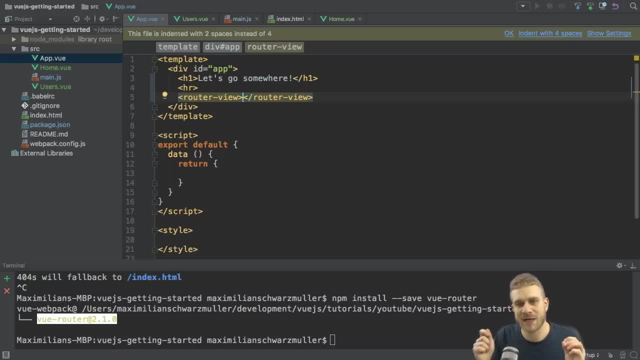 It looks like a component, right, And it will be recognized by the user, By the Vue router, And then it will take this place in our template And put the component which gets loaded conditionally And this place. So let's run the server again by running npm: run dev here. 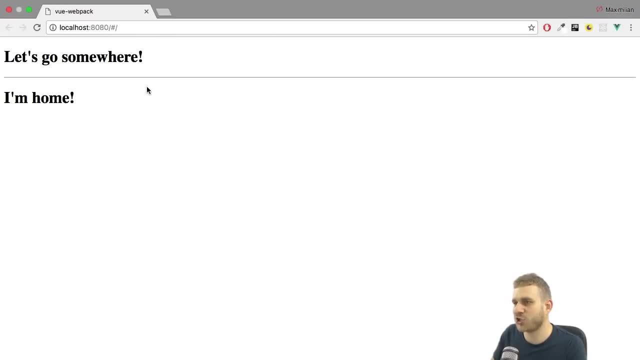 And we should have working routing now, If we go back to the application, Looks pretty good already We're at, I'm home Just by well loading our page, And we do recognize this strange hashtag here, right? Well, I'll come back to this in a second. 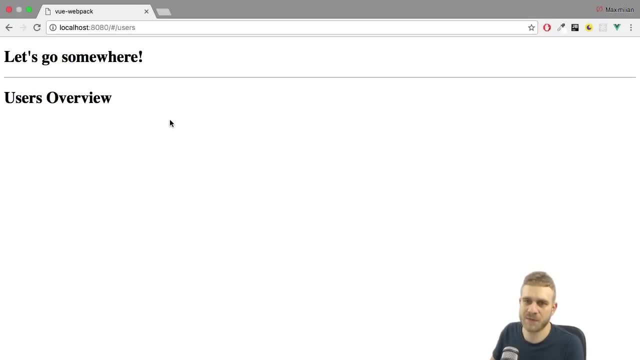 Let's try slash users again. Looks good to me, So that's getting loaded. Though, what is this strange hashtag here doing? Why can't we just visit slash users? Why is it always putting this strange hashtag here? And now it looks even weirder. 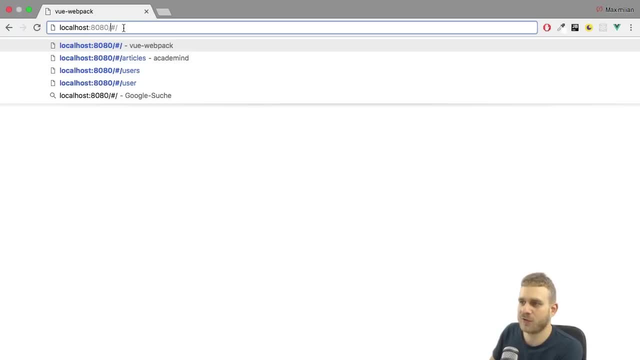 What's that? Well, this hashtag here, which gets added automatically, Is kind of the way how we did routing a couple of well years ago, One or two years ago even. It basically means The part in front of the hashtag. This part here gets handled by the server. 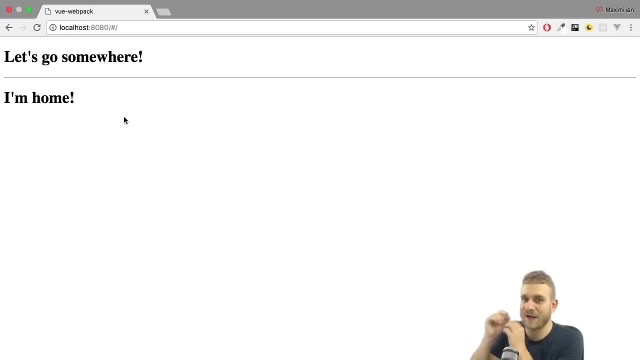 Because this is important. Every route or every URL you enter up here And when you hit enter Gets, of course, sent to the server. That's how the internet works right. It would be bad if it would be otherwise Or if it would work otherwise. 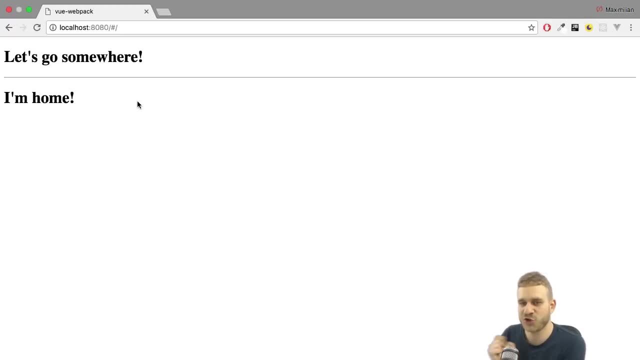 But here our routes are set up in our Vuejs application, Which of course runs in the browser. So how on earth Should our server know That there is a slash users route In our client application, In our Vue application? The answer is: it doesn't. 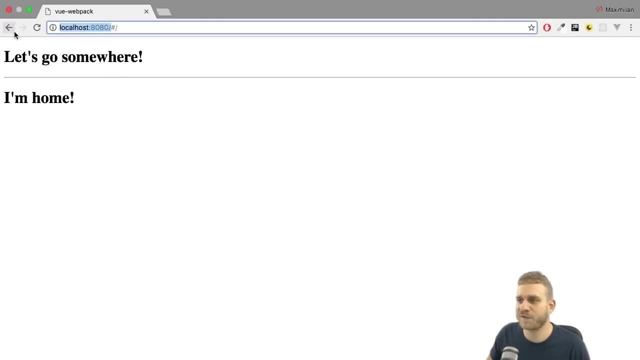 And this is where this hashtag here comes in. The part in front of the hashtag Is sent to the server And the server tries to find a fitting route. The part after the hashtag Is ignored by the server And instead handled by the client. 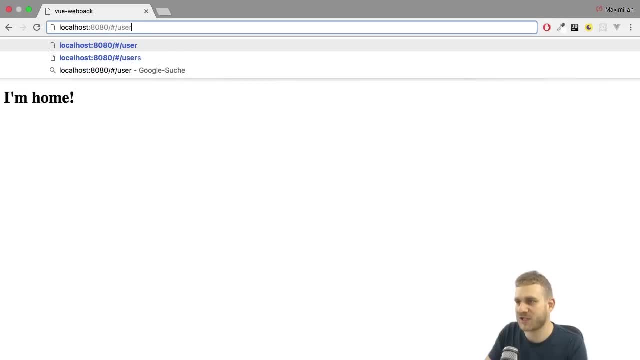 By Vuejs. This is why here we can enter slash users And we do load this route, Because the server Loads this part here, Gives us the index HTML page, The Vuejs application starts up And then this part here is sent to our 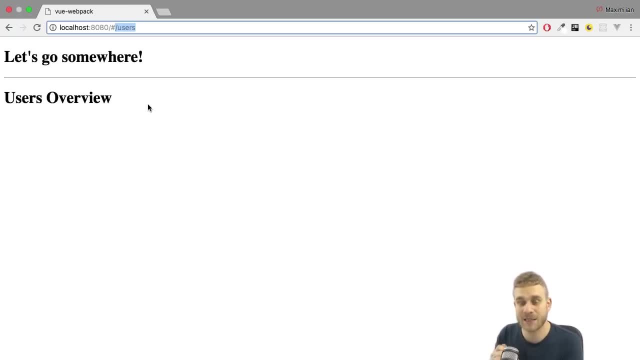 Frontend application to JavaScript And this is able to handle it Because we registered this route. Now that's nice, But you probably noticed, If I delete the hashtag and just enter Slash users, It now puts the hashtag here after users. 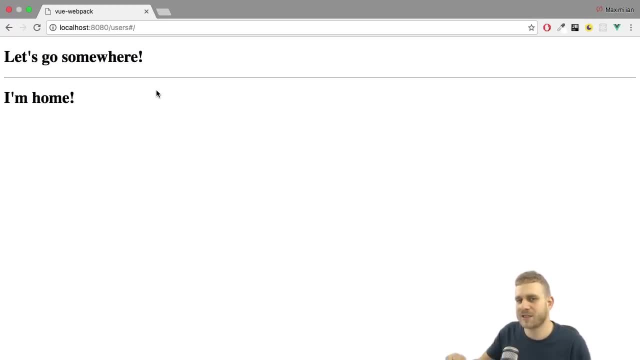 Well, that is because our test development Server here Is already configured in a certain way Where it will send all 404 errors, So every route it doesn't find on the server Automatically to the client. That is a cool behavior which you see a lot nowadays. 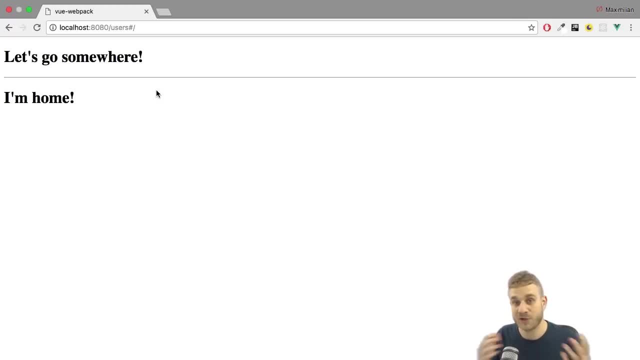 And you want to configure Your server in this way. Chances are. I want to do that, of course, At least Because if you do it like this, If you ignore all not found 404 errors on the server, You can always pass on. 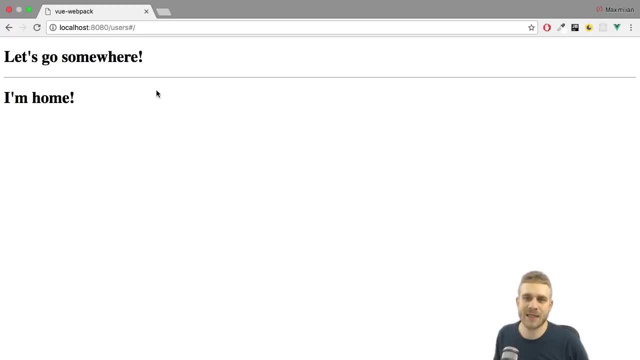 Unfound routes To the client And let the client handle it, Which is what we want to do here. Our server only has one route, Just the route route, This one here, So it should not even bother with any other routes. 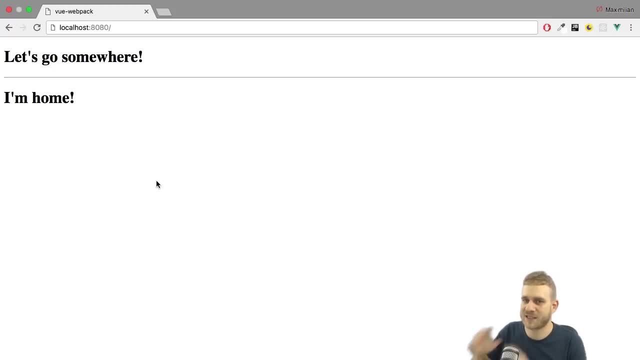 So we don't need the hashtag. We can tell it. Well, please always send all requests to the client. Now, as I said, this development server Is already configured in a way, Your server, Or the server you want to use for your application. 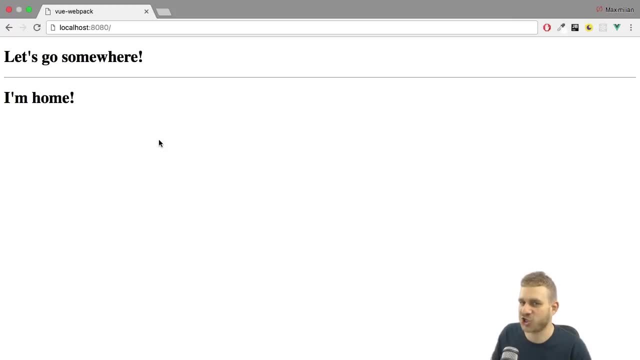 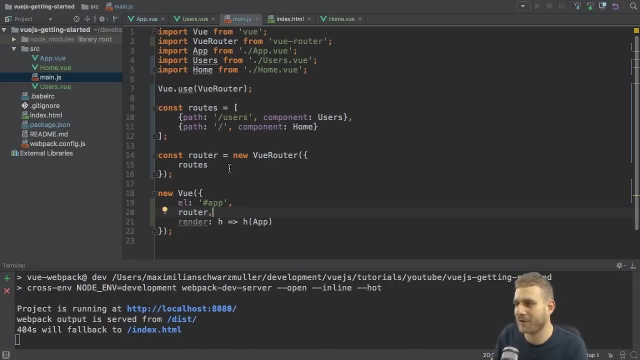 Has to be configured in such a way That it always sends back The indexhtml file. If that is the case, We can get rid of the hashtag By going to our mainjs file, To the router which we configured here, And adding the mode property.